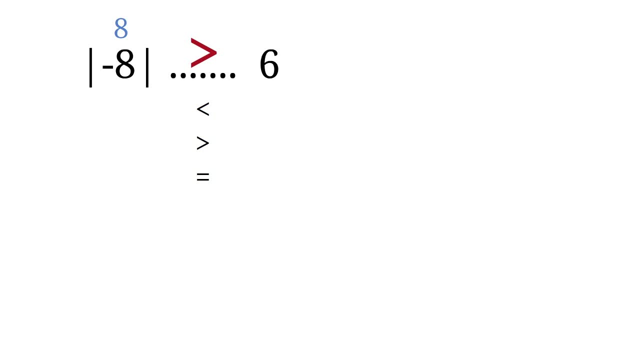 than 6.. I'm sure this was pretty easy for most of you. Now let's move on to the actual solving of absolute value equations. The absolute value of X is 2.. Find X. In our intro we got to know that the absolute value of negative 2 is 2, and also the absolute value of 2 is 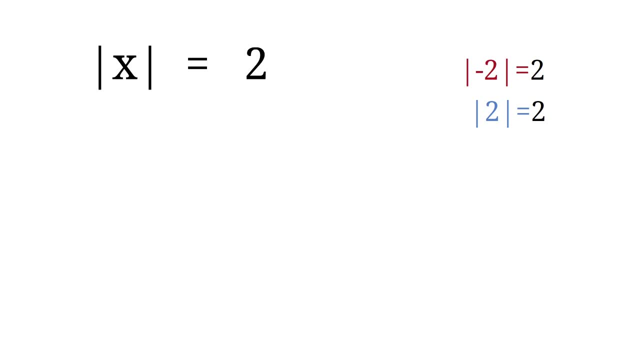 2. This means that for this question, the X value can be negative, 2 or positive, 2. Both of these will give 2.. What this implies is that to solve an absolute value equation, whatever is in the absolute value, in this case the X, is equal to the positive or the. 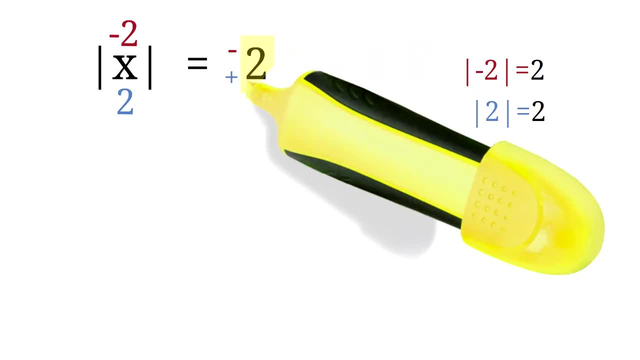 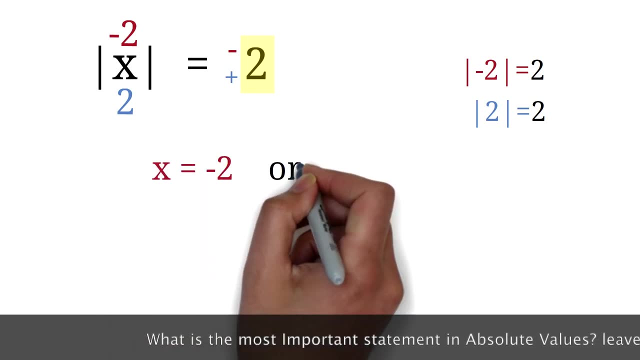 negative of what is on the other side of the equation, in this case the 2.. This is the second most important equation. This is the second most important statement in absolute values. So X equals negative 2 or X equals positive 2 for this question. Let's look at our next question to make this. 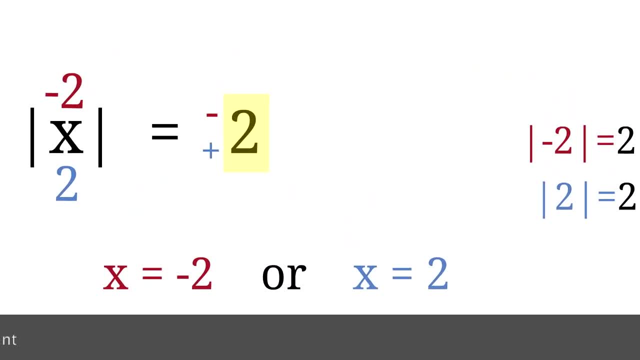 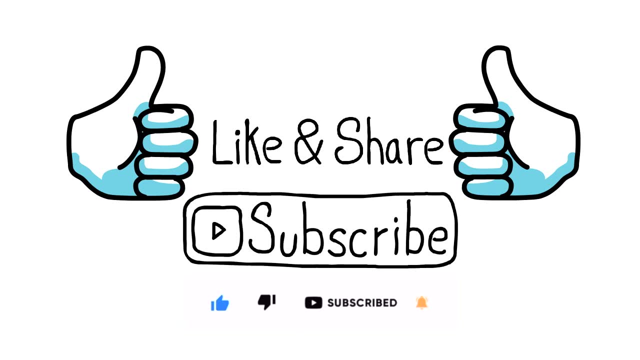 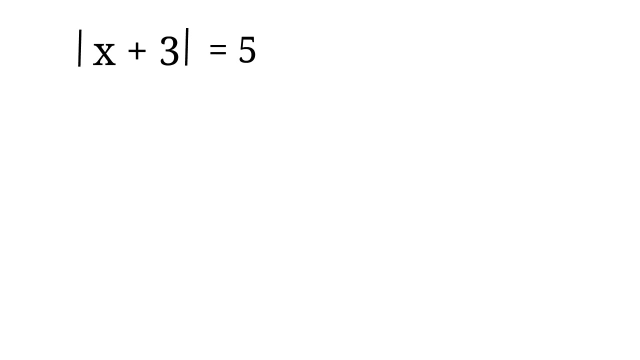 idea even clearer. Please encourage us to post more videos by liking, sharing and subscribing. We really appreciate it. The absolute value of X plus 3 is 5.. Find X. We said that whatever is in the absolute value- in this case the X plus 3, is equal. 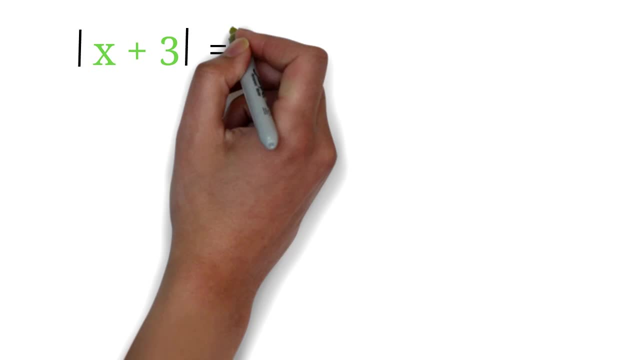 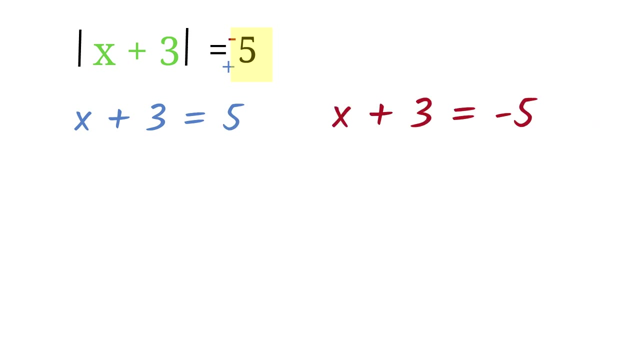 to the positive or negative of what is on the other side, in this case the 5.. So we can say X plus 3 equals 5, or X plus 3 equals negative 5. To find X we have to solve both equations. For the first one we will subtract 3 from both sides. The 3 will cancel out. 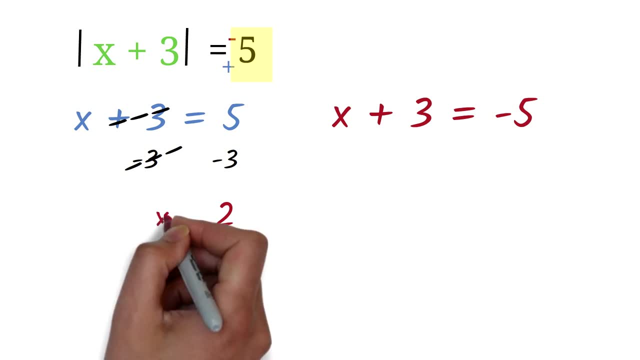 5 minus 3 is 2.. Therefore X equals 2.. For the second side, we will subtract 3 from both sides. The 3 will cancel out Negative. 5 minus 3 is negative, 8.. Therefore X equals negative 8. So X equals. 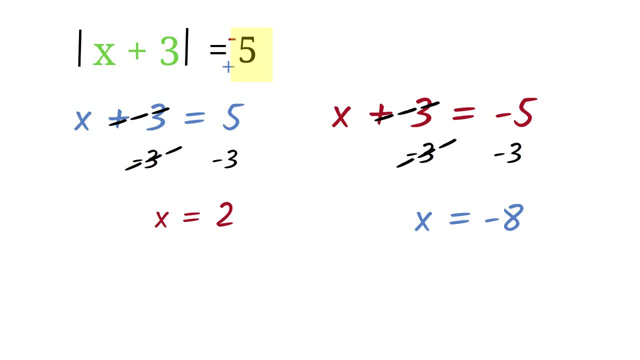 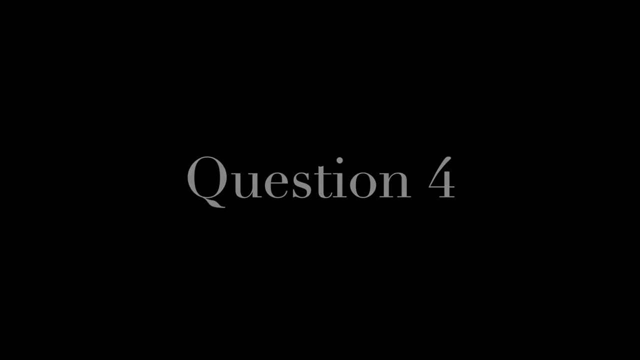 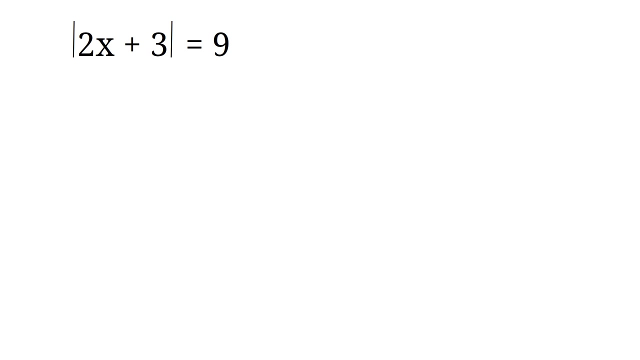 2 or X equals negative 8. for this question, The absolute value of 2X plus 3 is 9.. Find X: I'm sure we are familiar with what the steps are. We will equate 2X plus 3 to: 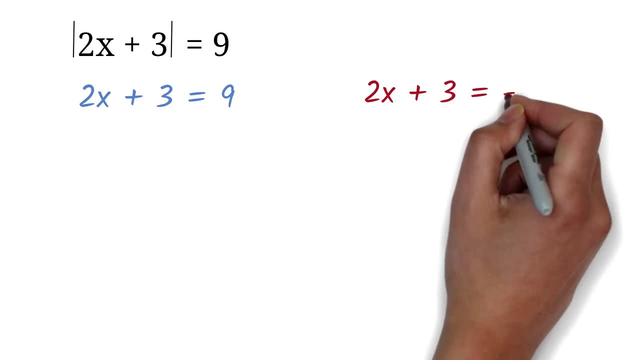 positive 9.. Then we will equate 2X plus 3 to negative 9.. From here, the work is your ability to solve equations. We have two step equations. We will subtract 3 from both sides. The 3 will cancel out. 9 minus 3 is 6.. We have 2X equals 6.. We will divide both sides. 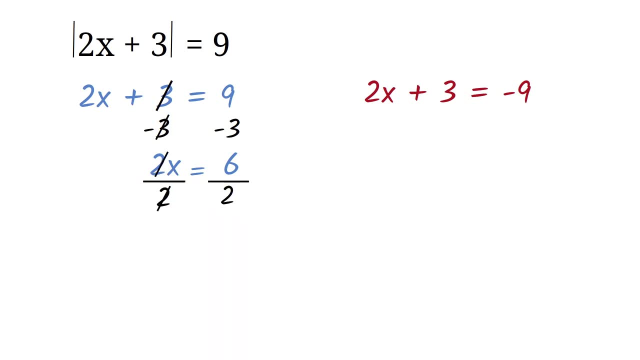 by 2.. The 2 will cancel out. 6 divided by 2 is 3.. So we have X equals 3.. For this side, we will subtract 3 from both sides. The 3 will cancel out Negative. 9 minus 3 is negative. 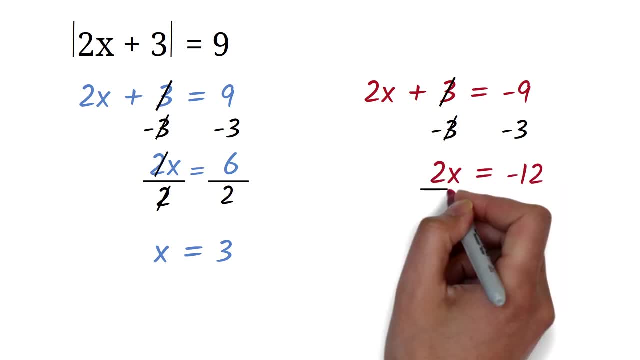 12. So we have: 2X equals negative 12. We divide both sides by 2.. The 2 will cancel out Negative 12 divided by 2 is negative 6. So X equals negative 6. Therefore X equals 3 or X equals negative 6.. 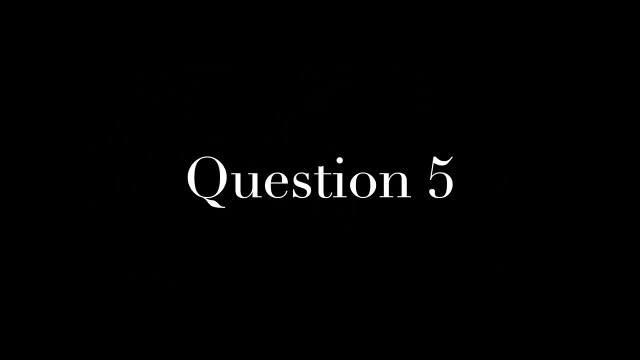 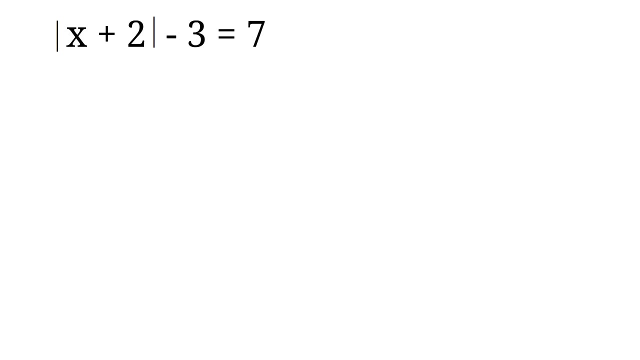 The absolute value of X plus 2, minus 3 is 7.. Find X. Here we will see that we have minus 3, which is not in the absolute value lines. We want only the absolute value to be on one side. When you have anything outside the absolute value, you have to get rid of it. So here: 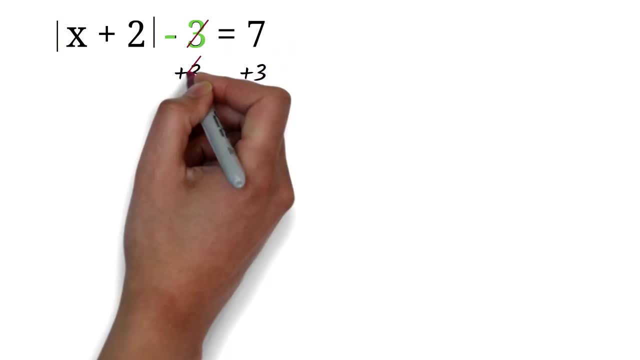 we will add 3 to both Sides of the equation. The 3 will cancel out. 7 plus 3 is 10.. So now we have the absolute value of X plus 2 equals 10.. We can work on this. now We have only. 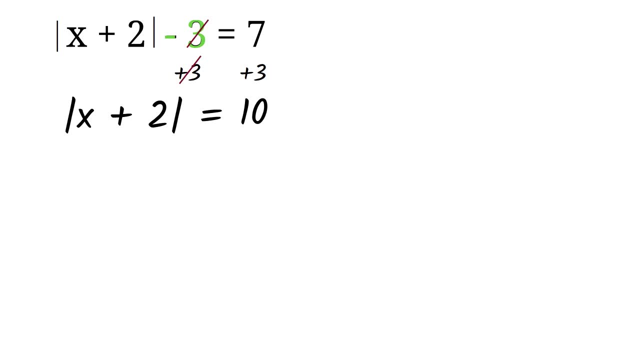 the absolute value part on one side of the equation. We said: in this case you will equate X plus 2 to positive 10, then equate X plus 2 to negative 10. For this part we will subtract 2 from both sides. The 2 minus 3 equals negative 12.. So we have aPs plus 2 minus 10.. Now we 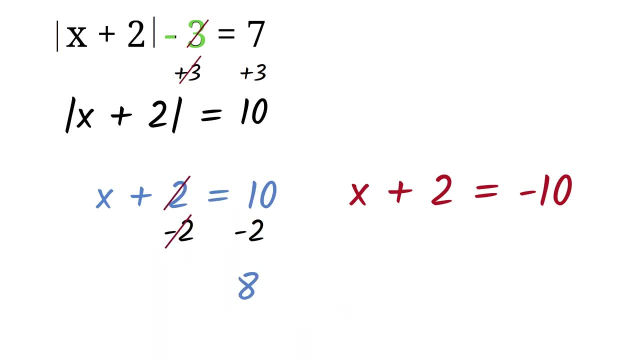 can solve over the 45th problem. The equation is as follows: When we leave the corner of the room, We put what is greater than the 90,000. We cut into a quarter off. added 2 will cancel out. 10 minus 2 is 8, so x equals 8.. For this part, we subtract 2 from both. 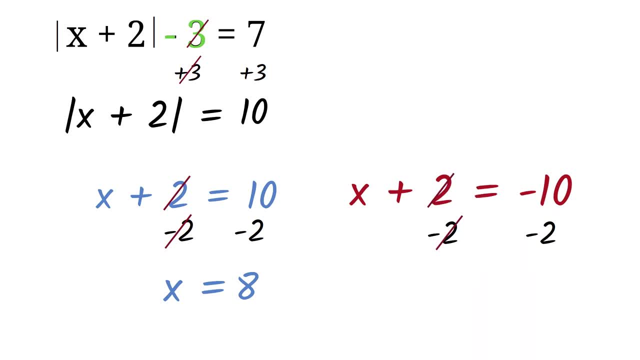 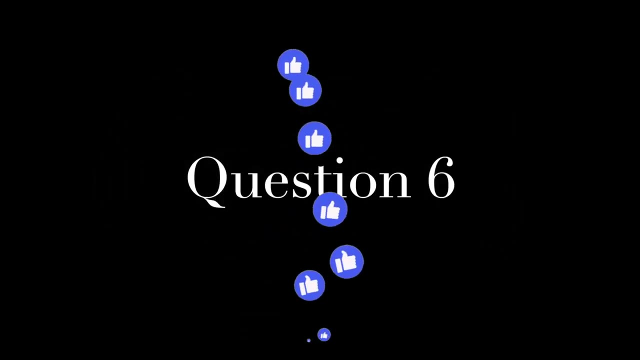 sides, The 2 will cancel out Negative. 10 minus 2 is negative 12. So x equals negative 12. Therefore x equals 8 or x equals negative 12.. The absolute value of 2x plus 4 is 6.. 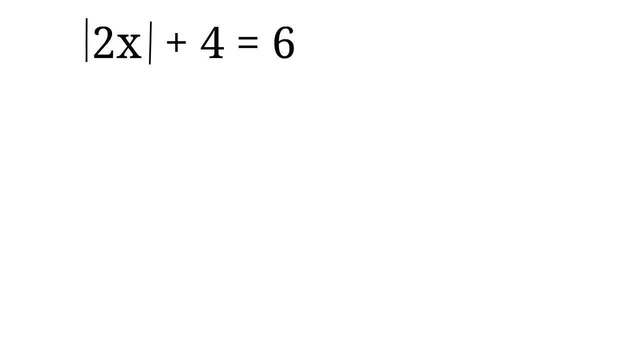 Find x. Please try this. It's just like the previous question. We want only the absolute value to be on one side of the equation, so we have to remove the 4.. We do that by subtracting 4 from both sides. The 4 will cancel out. 6 minus 4 is 2.. So the absolute value of 2x. 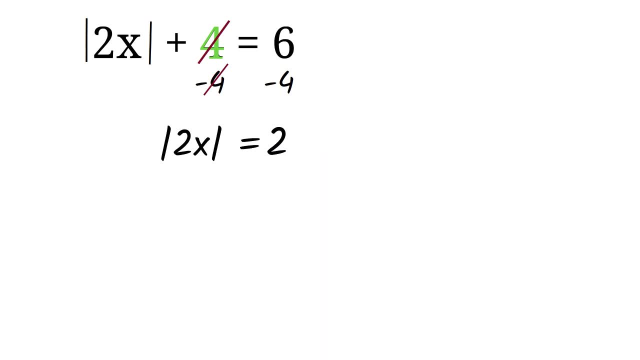 equals 2.. We have the absolute value on one side of the equation, so we equate the 2x to positive 2 and then equate the 2x to negative 2. We solve it, Divide both sides by 2.. The 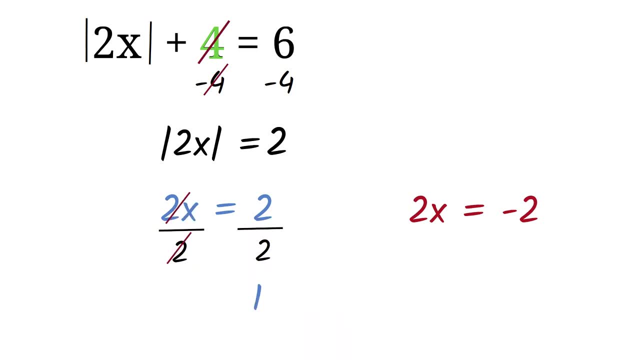 2 will cancel out. 2 divided by 2 is 1.. Therefore x is 1. here Again, we will divide both sides by 2.. The 2 will cancel out Negative. 2 divided by 2 is negative, 1.. So x equals. 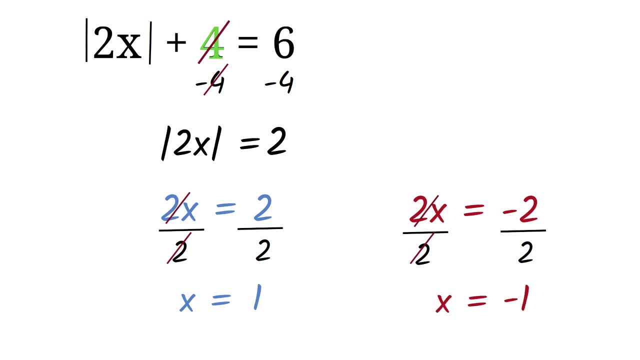 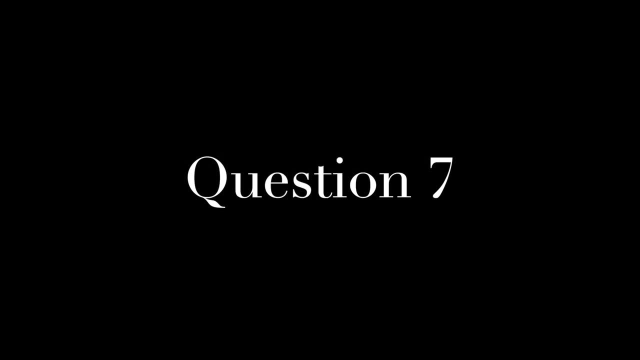 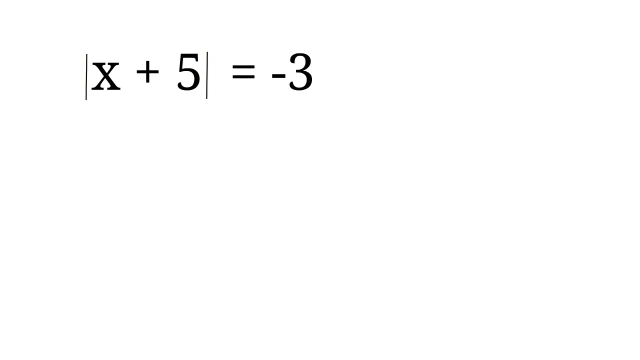 negative 1.. Therefore, x equals negative 1 or x equals 1.. The absolute value of x plus 5 is negative. 3. Find x. This question is very important. One thing we should know is that the absolute value cannot be negative. So if you have absolute value on one side, 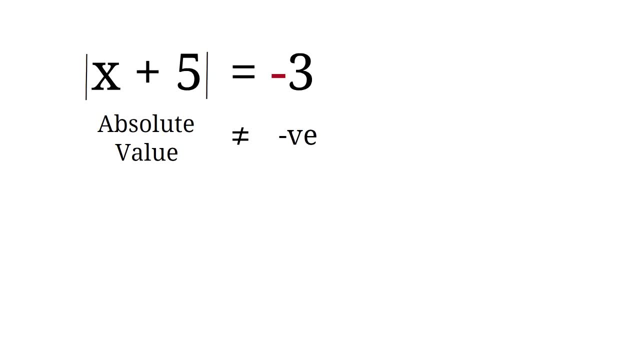 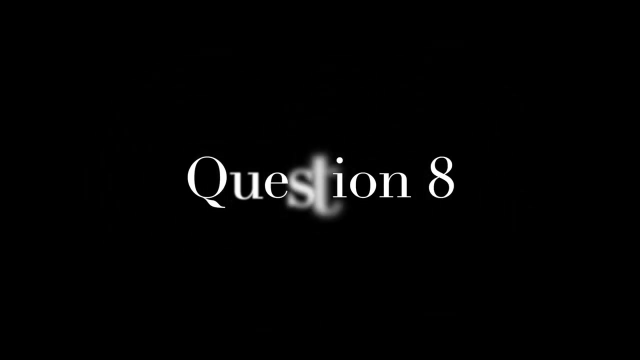 then the other side cannot be negative. We say that this has no solution. When you have the absolute value on one side of the equation and negative on the other side, it has no solution. The absolute value of x plus 5 minus 5 is negative. 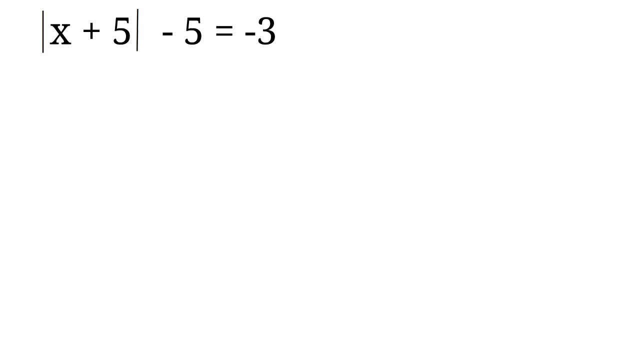 The 1 is negative. 3. Find x. This question is also very important because we want you to know that you should not automatically assume that a negative on one side of the equation means there is no solution. You have to make sure that only the absolute value. 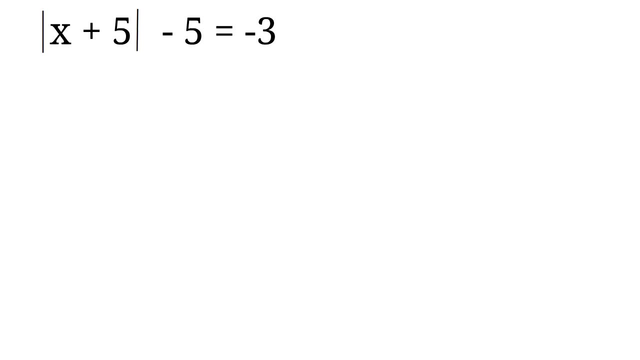 is on the other side. So here we know. our first step is to get rid of the negative 5. We do that by adding 5 to both sides of the equation. The 5 will cancel out Negative. 3 plus 5 is 2.. Therefore, x equals 2 is negative 3. We try to eliminate x plus 5.. So when we 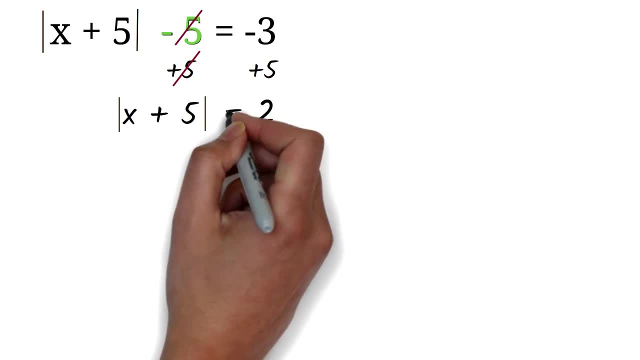 is 2.. We have the absolute value on one side, but we can see that we now have a positive 2 on the other side. So this has a solution. We solve it: x plus 5 equals 2, or x plus 5 equals negative 2.. 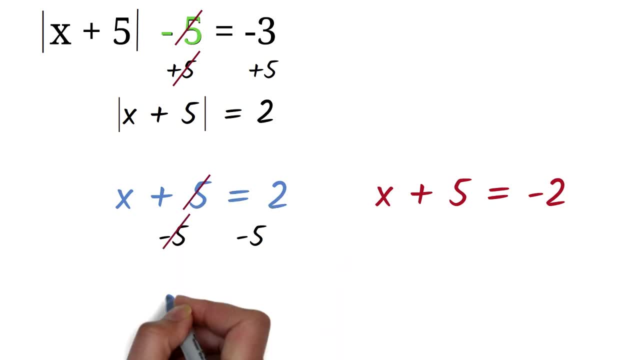 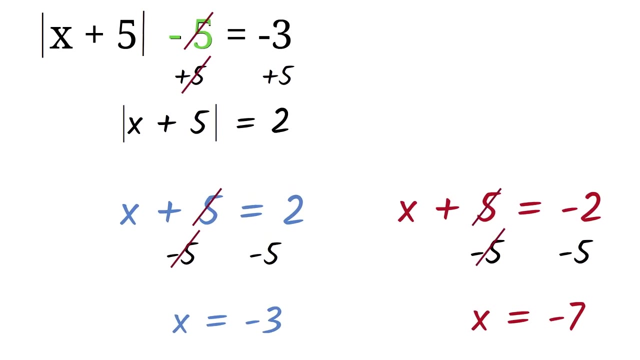 Subtract 5 from both sides, We will get x equals negative 3. Here again, we will subtract 5 from both sides to get x equals negative, 7. So x equals negative 3 or x equals negative 7.. The absolute value of 2x plus 5 equals x minus 7.. Find x. Here we are looking at the situation. 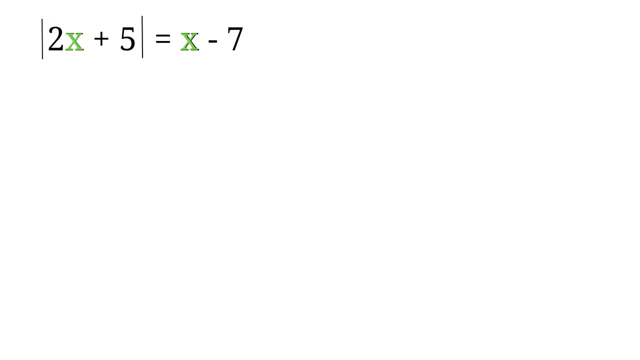 where there is x on both sides of the equation. Please, this question is extremely important. Let's look at the situation where there is x on both sides of the equation. Let's exercise our brain. We will start with our usual process. We will equate 2x plus 5 to x. 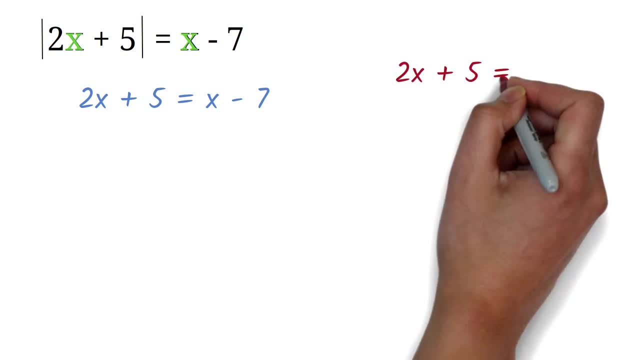 minus 7.. Then we will equate 2x plus 5 to negative x minus 7.. Notice I put this in parenthesis. This is to make sure we distribute the negative on both the x and negative 7.. We want to get the x. 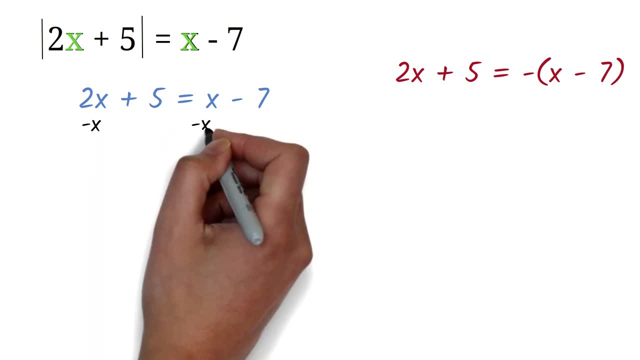 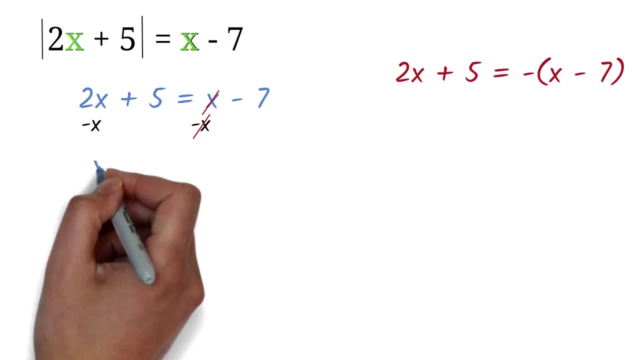 on one side of the equation. We will subtract x from both sides. The x will cancel out 2x minus x is x, So we have x plus 5 equals negative 7.. We can now subtract 5 from both sides, The 5. 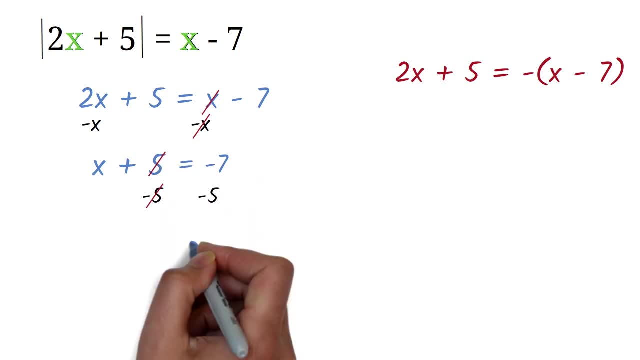 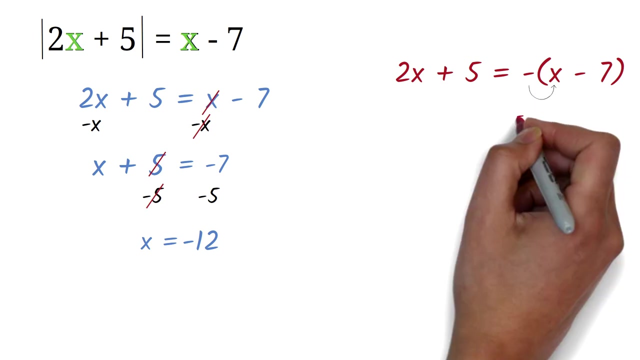 will cancel out Negative. 7 minus 5 is negative 12.. So x equals negative 12.. Now we work out this side. We will first distribute the negative. This is really the same as negative 1.. So negative 1 times x is negative x, And negative 1 times negative 7 is x. So we have x plus 5 equals. 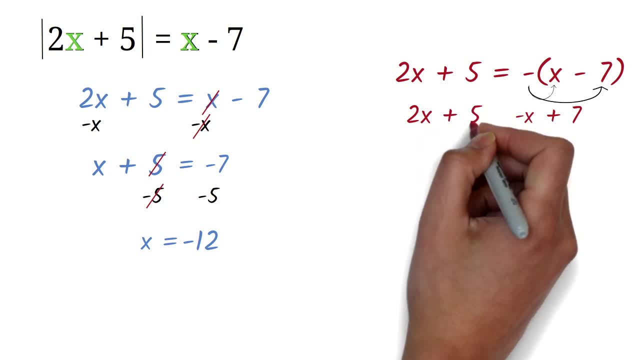 7.. So we have 2x plus 5 equals negative x plus 7.. We go through the same process again. Add x to both sides. The x will cancel out. 2x plus x is 3x. So we have 3x plus 5 equals 7.. Now we subtract. 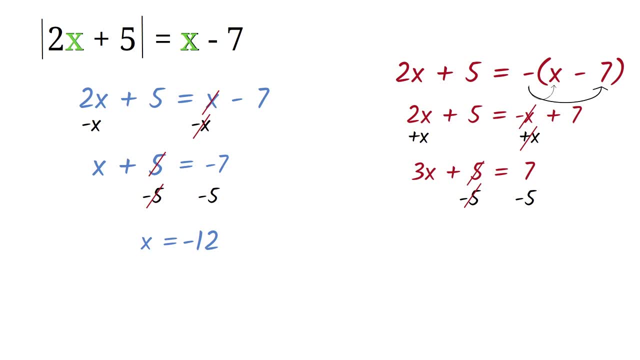 5 from both sides. The 5 will cancel out. 7 minus 5 is 2.. We have 3x equals 2.. We divide both sides by 3.. The 3 will cancel out. 2 divided by 3 is 2 over 3.. So we have x equals 2 over 3.. Now here is. 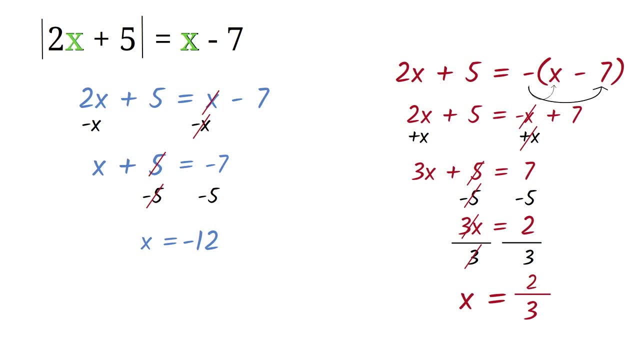 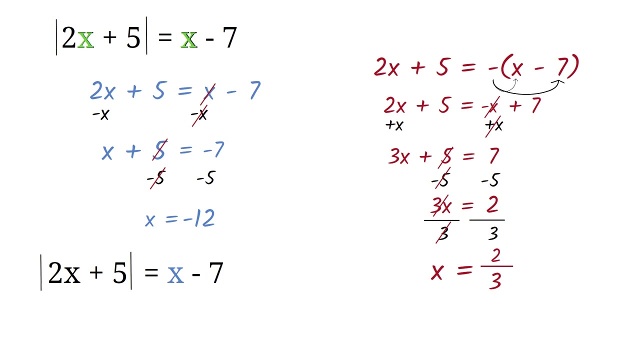 where it gets tricky: When you have the absolute value on one side and the other side has an x value or variable, you will have to substitute each value to check if it satisfy the idea that the absolute value cannot be negative. Let's write our question down here so we can easily use it. 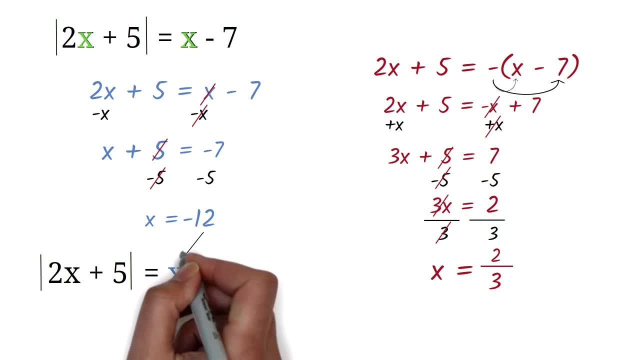 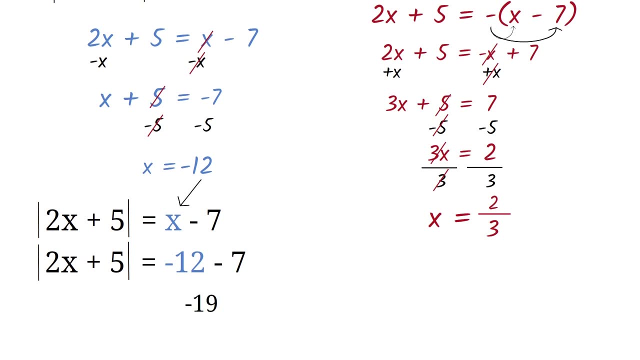 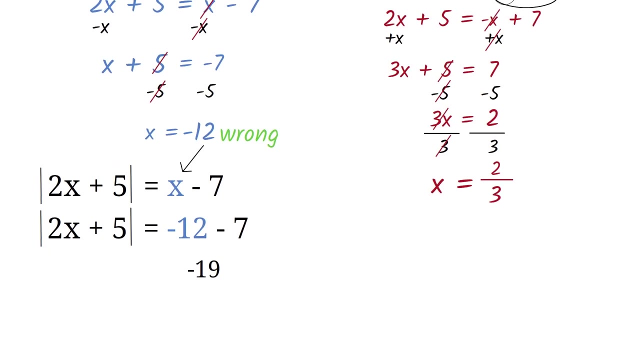 We will replace the x, We will get the absolute value equals negative 12 minus 7.. This will give us negative 19.. Since the absolute value cannot be negative, this x value does not satisfy the equation. We work with the 2. 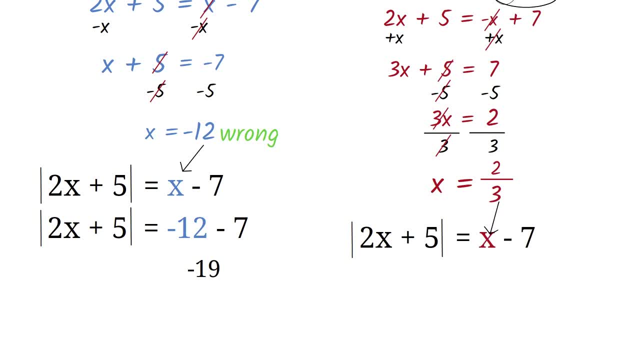 over 3.. We replace the x 2 over 3 minus 7 will give us negative 6.33.. This is also negative. We know the absolute value cannot be negative. Since both x values gave us a negative value, we can say this has no solution. Please take. 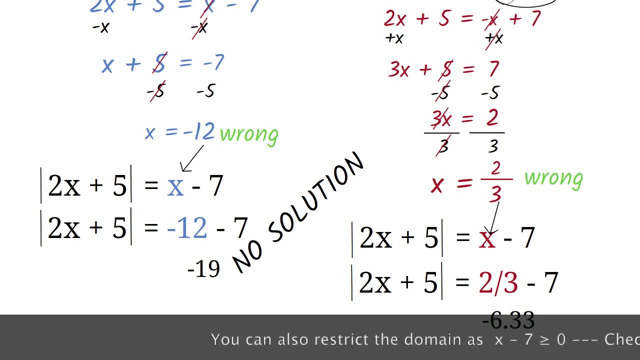 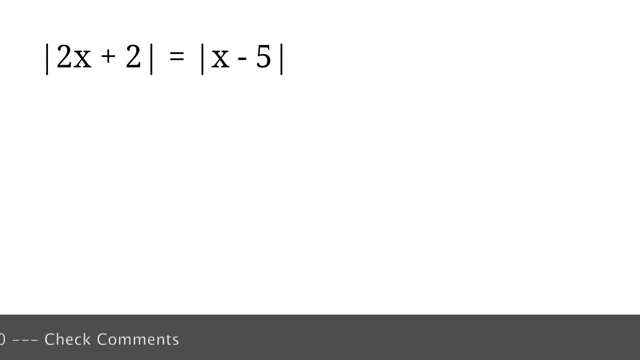 note of this. It is one of the hardest version of this kind of absolute value equations. The absolute value of 2x plus 2 equals the absolute value of x minus 5.. Find x. Here we have absolute value on both sides of the equation. 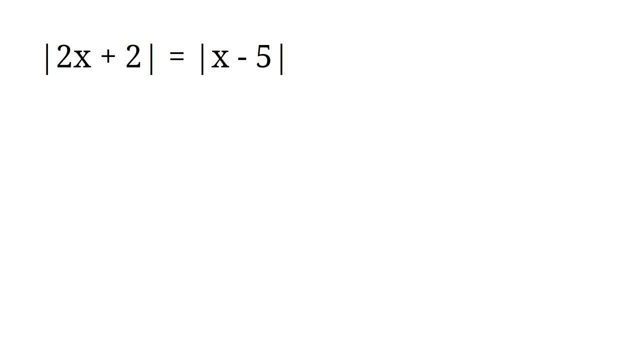 What we have to do is to remove the absolute value from one side and solve it like we have been doing. So I will have absolute value of 2x plus 2 equals x minus 5.. From here, it's just like what we've been doing. We will equate 2x plus 2 to x minus 5.. Then we will equate 2x plus 2 to